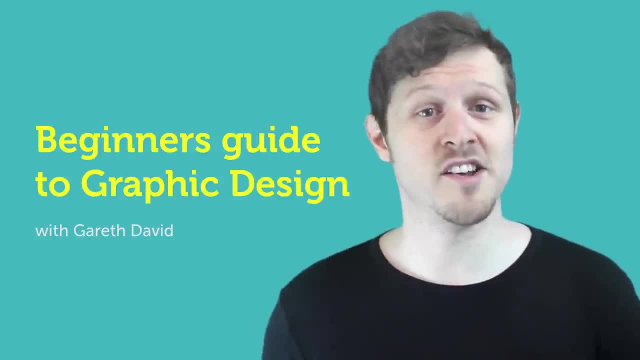 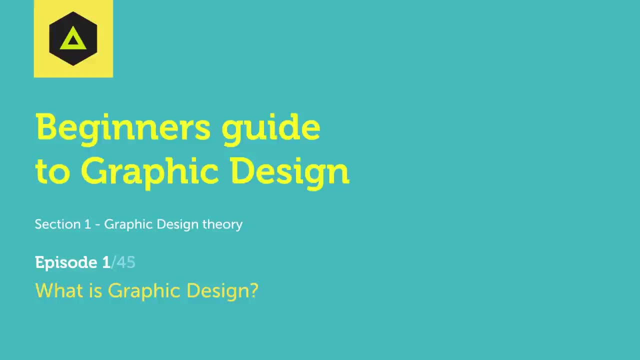 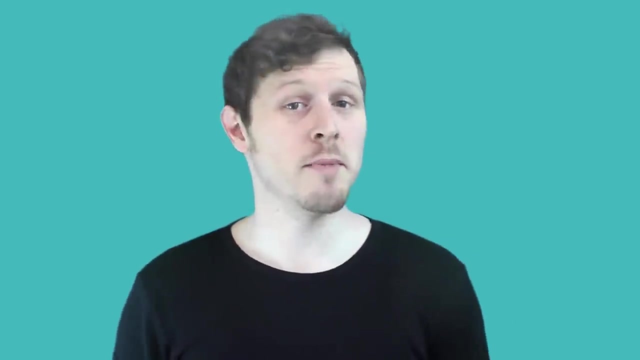 becoming a graphic designer, then join me as I discuss a series of graphic design topics. So you're interested in graphic design, perhaps considering becoming a graphic designer and looking to learn more. In this video, I'm going to discuss what graphic design is. Now a lot of. 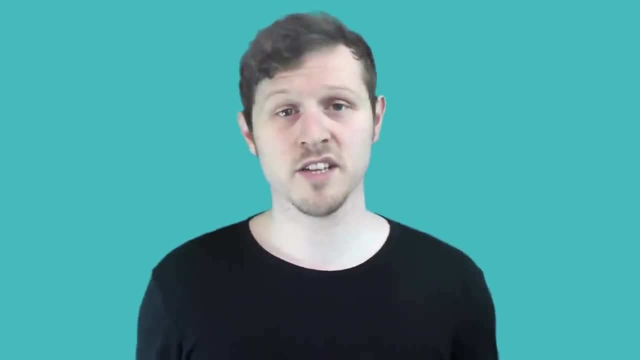 people on my channel have asked me this question, mainly youngsters and people who are thinking about pursuing graphic design and want to know what graphic design is and if it's right for them. Now, I have often found this a really hard question, as it does not. 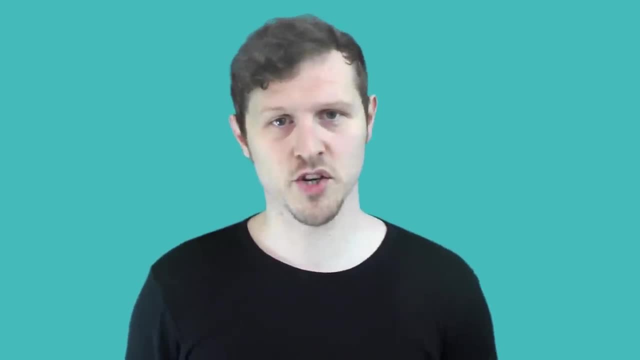 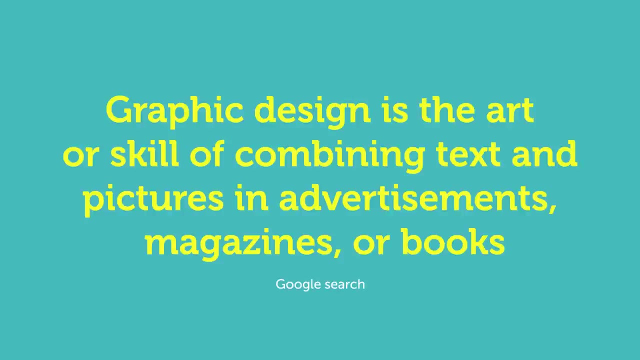 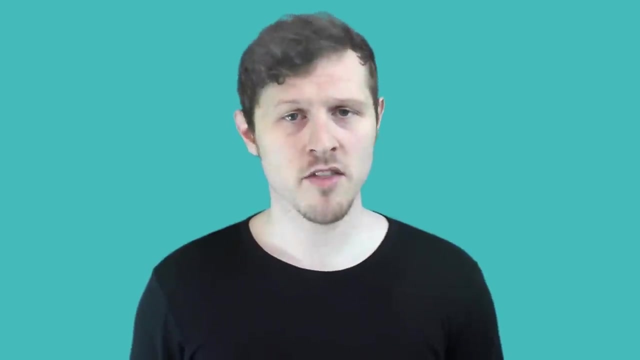 really have a simple answer without some degree of explanation. Now, if you google this, it will tell you that graphic design is the art or skill of combining text and pictures in advertisements, magazines or books. So quite a simple and accurate explanation there, though I happen to think. 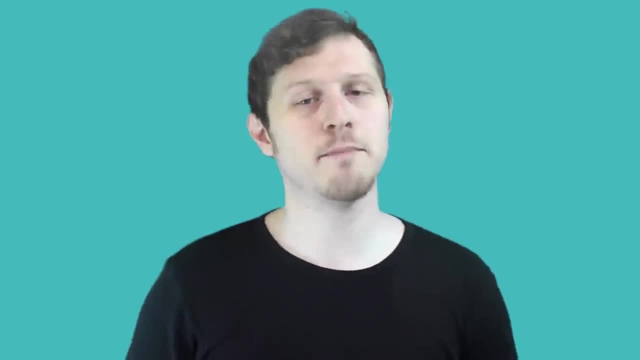 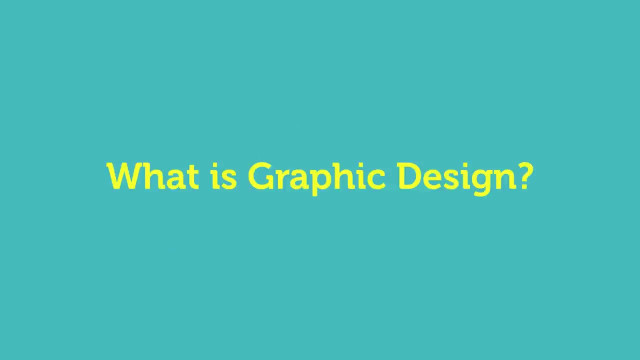 there's more to it than that. In this video, I'm going to attempt to answer this question and give you my take on it from my experience. So what is graphic design? Well, let's start simple. So, with graphic design, we have two things. we have graphic and design. Graphic is visual. 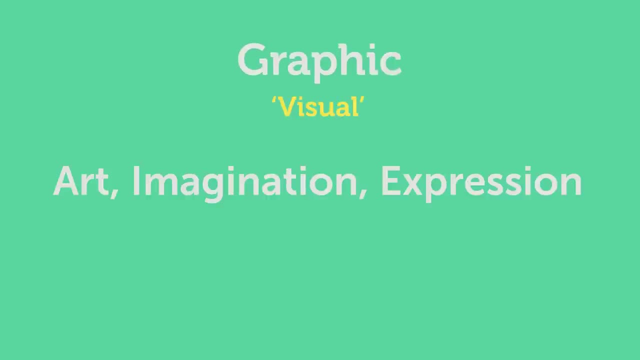 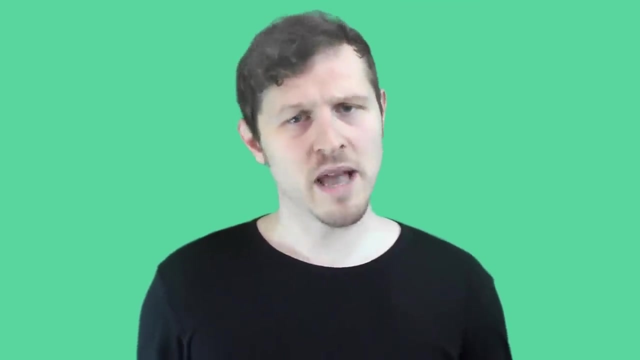 which is associated with art, imagination and expression, involving many mediums such as drawing, painting, engraving or lettering, given clear and explicit detail. So the graphic part of graphic design is made up of visual elements, the building blocks of design, The basic visual elements that combine to create graphic design include the following: 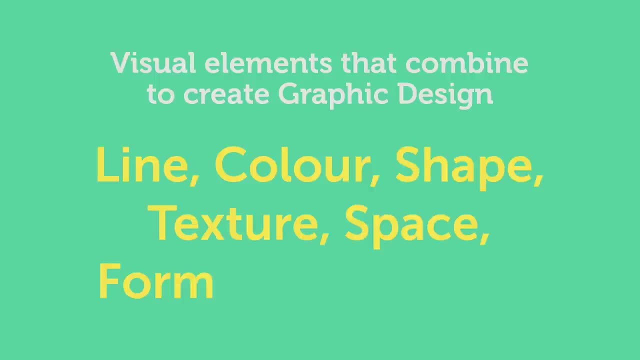 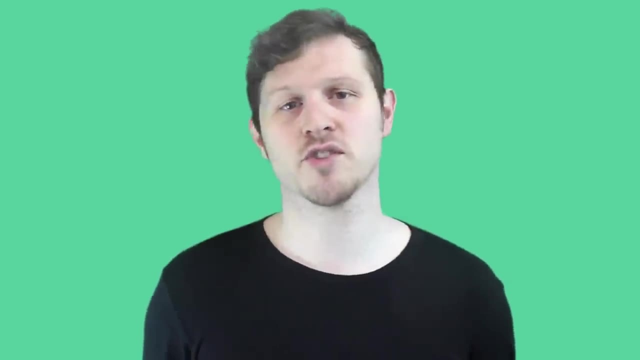 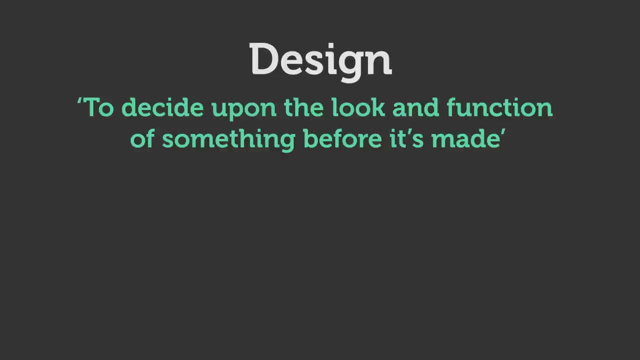 colour, shape, texture, space, form and typography. Through the harness of our artistic expression, we choose these visual elements and arrange them on a surface in a layout to convey an idea. Now the second part is design, which is to decide upon the look and function of something before it. 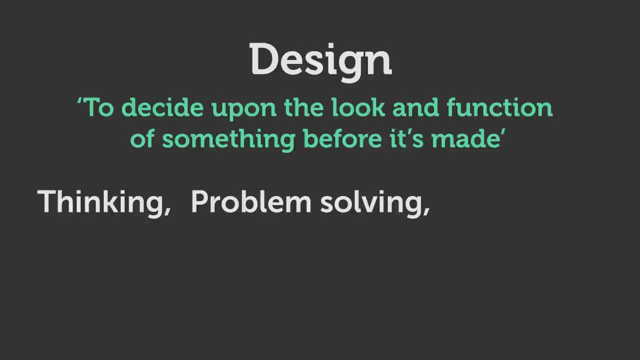 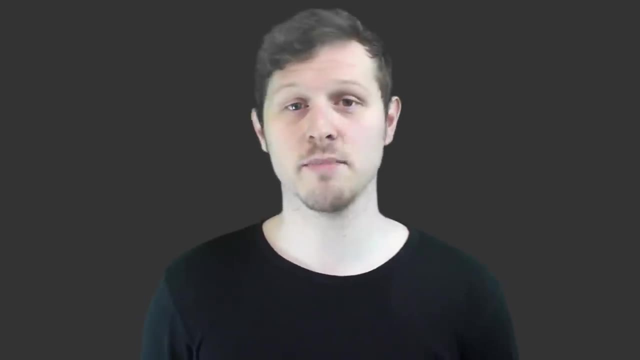 is made. So design is thinking, problem solving and practicality theory. In graphic design, there are rules that can be considered. These rules are called the principles of design. These principles all have a relationship between each other and appear in every well-designed piece of work, you see. So the design principles. 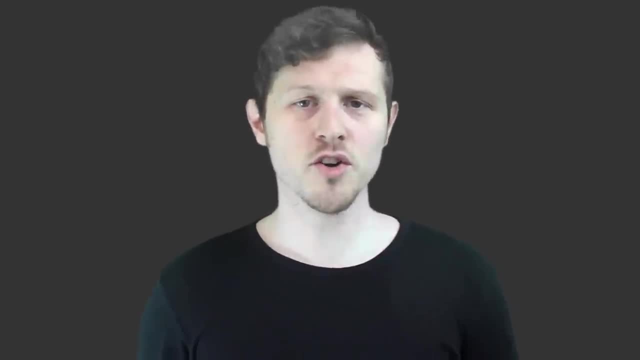 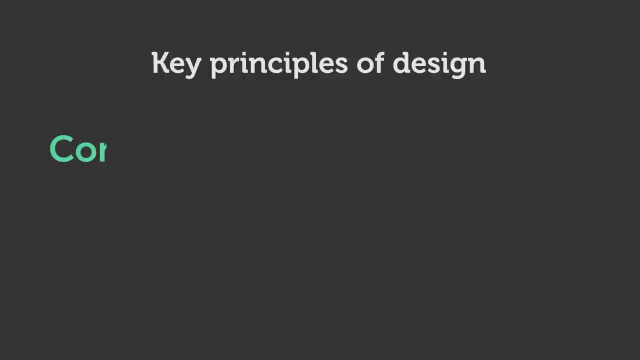 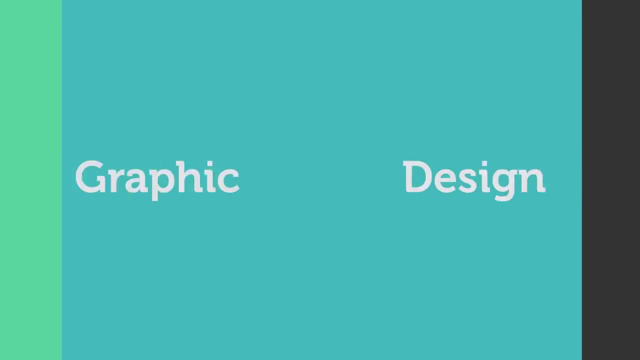 make the design in graphic design. A good grasp of design theory will mean there is always substance behind your work. The key principles of design are contrast, hierarchy, alignment, balance, proximity, repetition, simplicity and function. When we bring both the visual elements and the design principles together, we have graphic design. 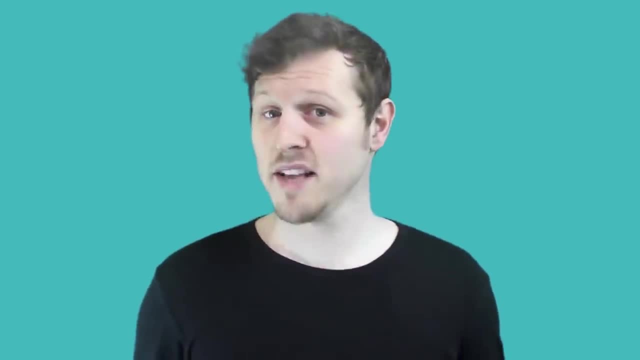 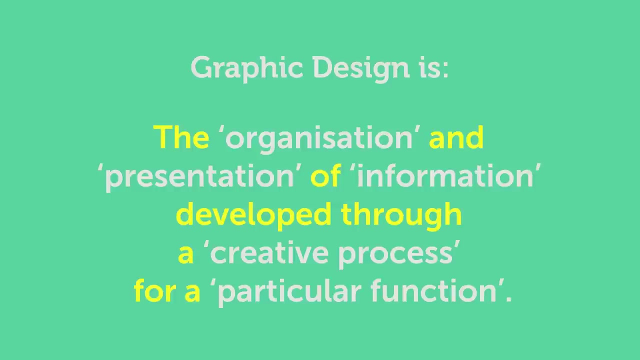 Now, graphic design is not drawing. graphic design is not painting. graphic design is not creating a poster or a quick logo on your computer. These things are the means to the end and skills in their own right. Graphic design is not about making things look pretty. Graphic design is the. 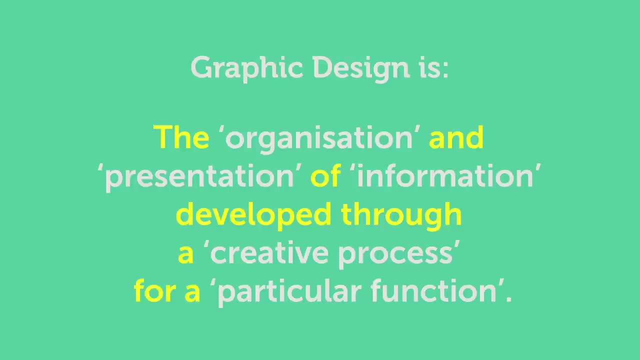 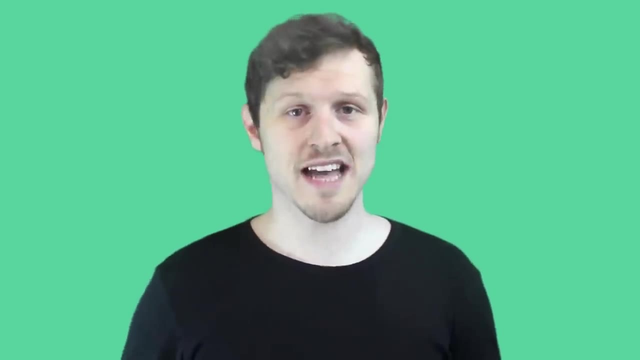 organization and presentation of information developed through a creative process, for a person, a particular function In graphic design, we must first understand information, a message or a brief- and then research, think, imagine and develop and create a solution, A concept, in order to 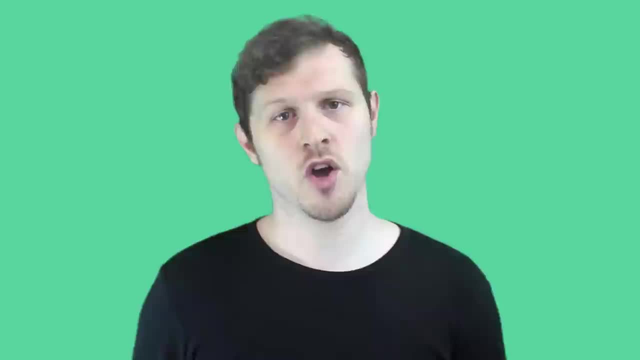 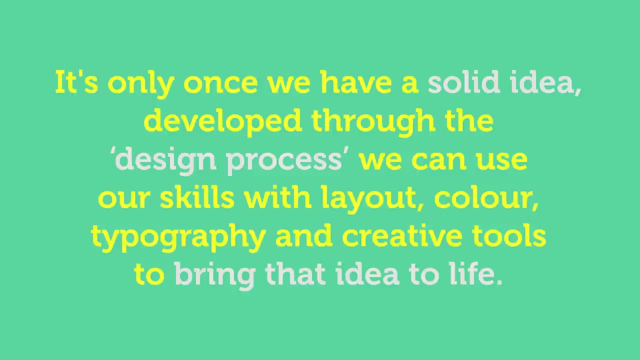 communicate that information, tell a story, a message or idea in a visual way. It's only once we have a solid idea developed through the design process, we can use our skills with layout, color, typography and creative tools to bring that idea to the next level. It's only once we have a solid idea developed through the design process, we can use our skills with layout, color, typography and creative tools to bring that idea to the next level. 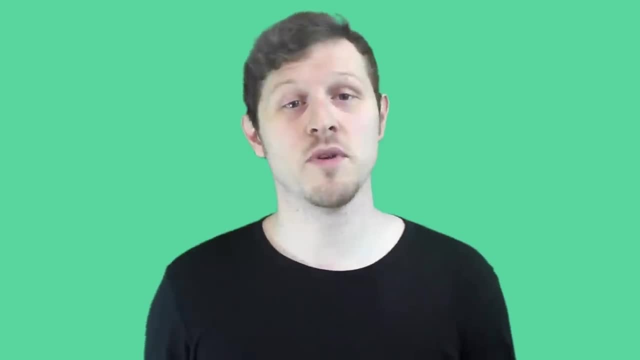 to life. Once upon a time, that would have been with just the aid of a pencil or a paintbrush on paper. Today, it's all those things and more. Today, we also have cameras, computers and printers, Since the invention of the print press, which enabled reproduction on a mass scale. 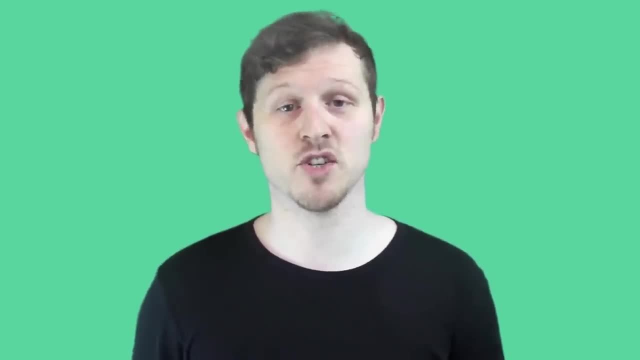 graphic design has been used to communicate and spread messages worldwide Through the evolution of technology. today, we are surrounded by an abundance of visual communication. Today, we are surrounded by an abundance of visual communication. Today, we are surrounded by an abundance of visual communication. graphic design is implemented across a broad spectrum of media, both print and digital. 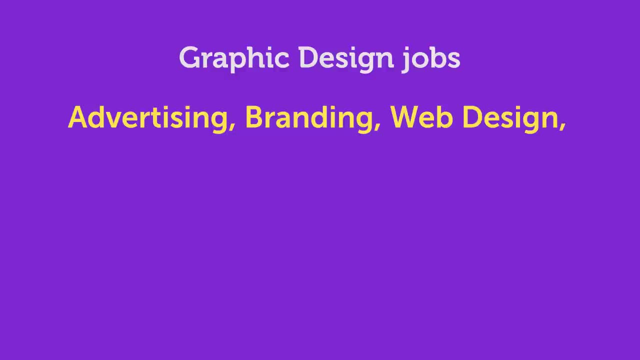 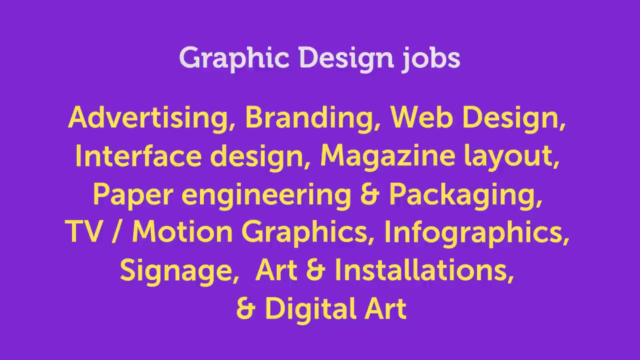 such as advertising, branding, web design, interface design, magazine layout, paper engineering and packaging, tv, motion graphics, infographics, signage, art and installations and digital art. If you are looking to pursue a career in graphic design, you will inevitably end up creating work.